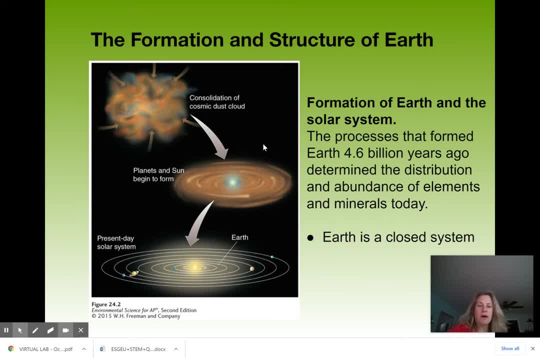 And then the rest is forming the planets. So this is the most concentration. So 99% of the gases are found within the center, which would be our center of gravity, which in every system would be a star. So in our case, 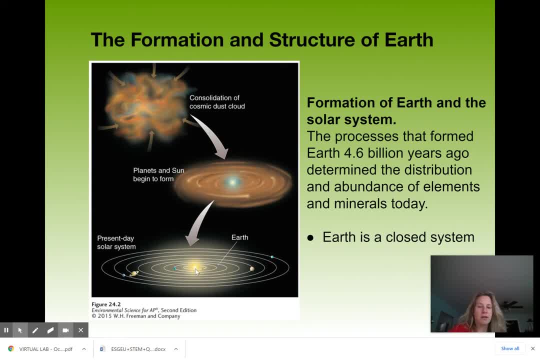 this is the solar system, So this is the star, the sun in the center, and then earth out here, And then, of course, like I said, the other planets, And then we've got all different kinds of other star systems that have formed planet systems as well, And so this is about 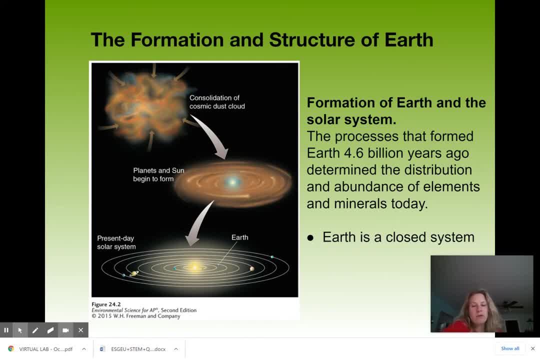 4.6 billion years ago And we can look at the rock record and we can date the rock back that far, So we can use things like uranium dating radon. let's see that's about the main things to date that far back would be using. 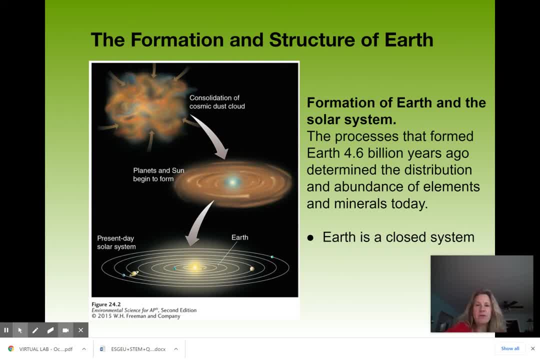 those things, And that's radiometric dating, So we can look at the half-life of those elements and we can figure out how long it's been since they formed, And so we can see the earth, Mars, the moon. all of those are about 4.6 billion years old. And just a reminder: earth is a closed 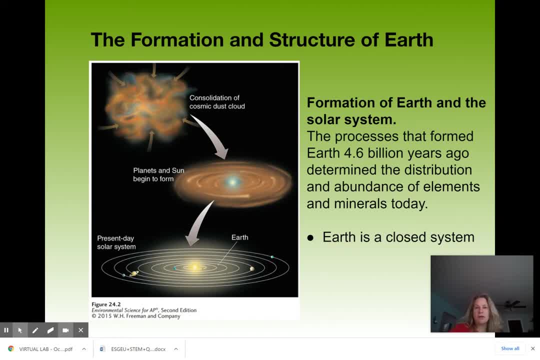 system, meaning that things don't enter and leave. So think about what that means for resources. So if it's a closed system, that means that all the resources that are available for humans are found on the earth right now, So we have no other resources outside of the earth that we can. 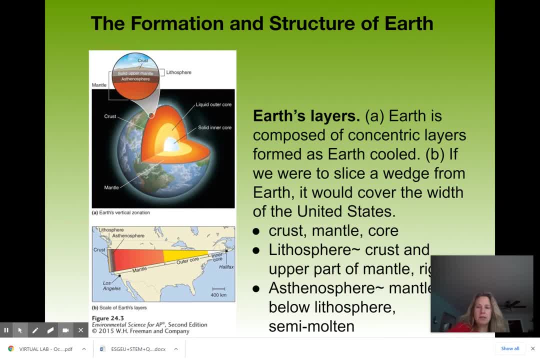 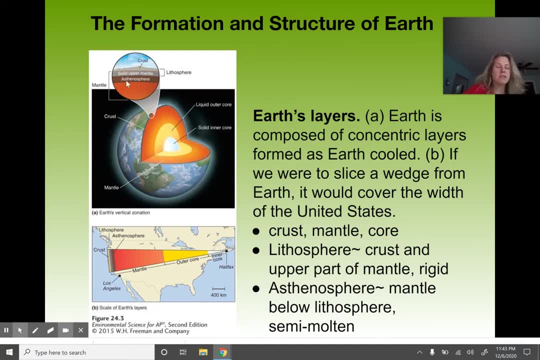 readily use, All right. So if we look at the earth in the structure, so we've got different layers of the earth. So, looking at the crust, going inward, we have the crust, then we have the upper part of the mantle which makes up the lithosphere. 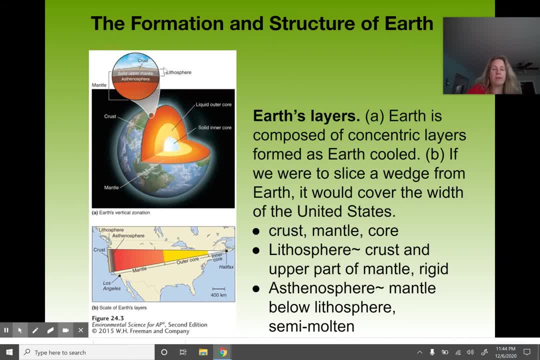 And so the lithosphere are the plates. You've probably heard of plates sliding around. So lithosphere is the plates, So crust and upper part of the mantle, And then we've got something called the asthenosphere below, And then below that we've got the upper, I mean. 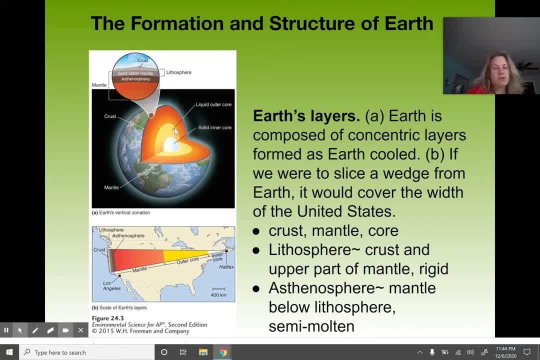 outer and inner cores, And so that's our layers. And then if we look at the depths of these, so they're comparing this to the US here. So here's the crust, And remember, the lithosphere is the crust and upper part of the mantle, And then we've got the asthenosphere, which is kind. 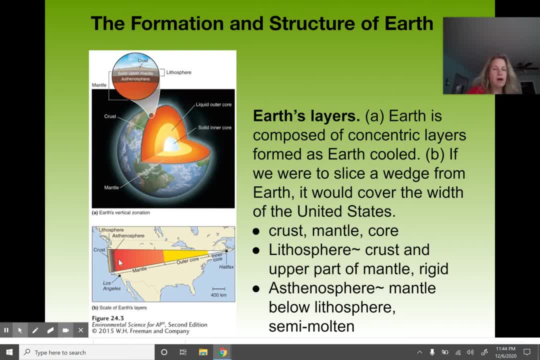 of like the middle small portion of mantle And then we've got the main mantle which makes up all of this. So basically, right below the crust, all the way to the outer core, is the mantle And then you've got the outer core, inner core. So this space, the spacing represents about the 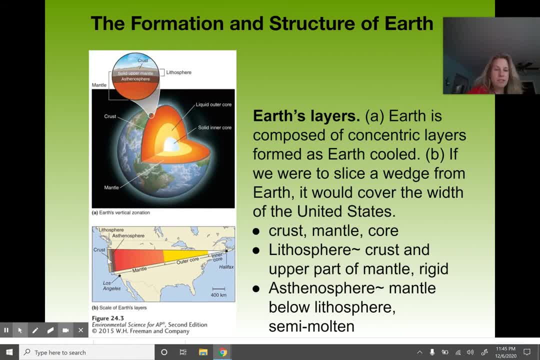 width of the US, And so you can see, if we were to dig down from the crust, we would be digging down through the entire US down to the core. So that would be pretty far. So just be familiar with these things. Like I said, this is a lot of earth science, but we need to talk about it because 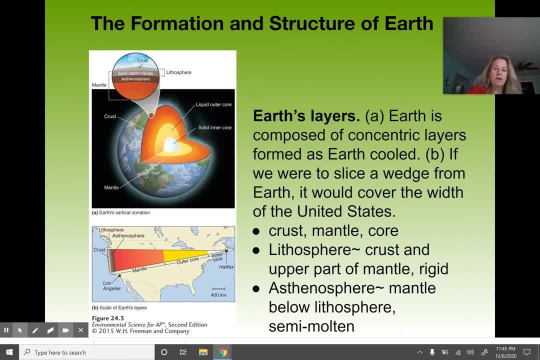 we're going to talk about resources, And so resources come from the earth. But we've got the crust, mantle, core, lithosphere, asthenosphere, So just be familiar with those terms and where they're located. All right, So we've got something. 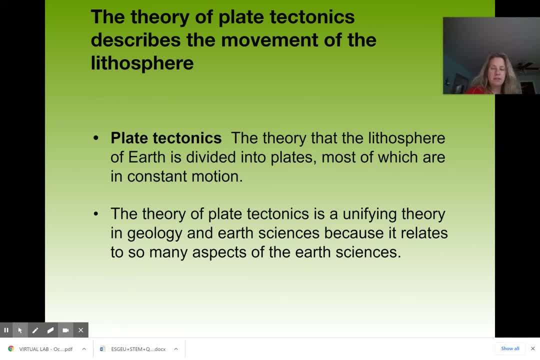 called plate tectonics, which is, like I said, the lithosphere, which is the crust and upper part of the mantle. Those are sliding around on the asthenosphere and they're colliding and moving apart and doing all kinds of things And that's creating volcanism. 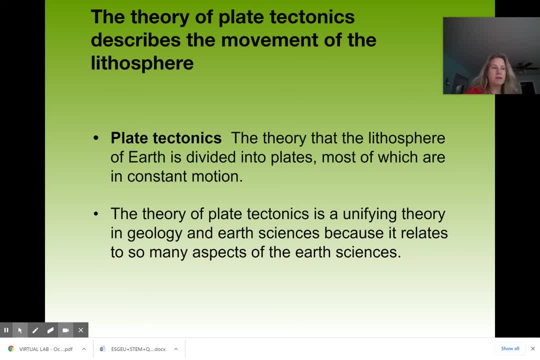 That's erupting, That's causing earthquakes, It's causing minerals to come to the surface that maybe otherwise didn't, So it's creating a lot of different things, But that's the theory of plate. tectonics basically states how that is occurring, So how the mantle is convecting. 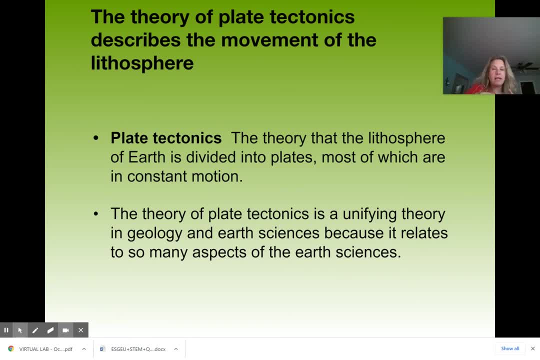 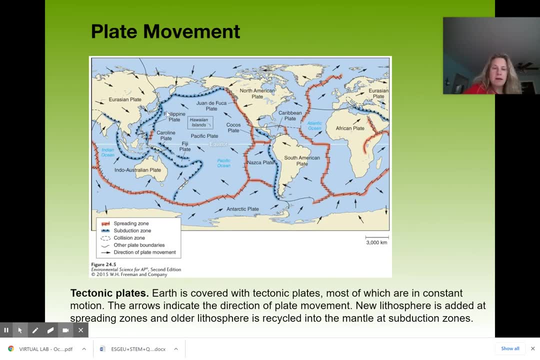 and the lithosphere on top of it is moving around and colliding and subducting and forming volcanoes and all kinds of things, All right. So here's our list of things, Our plates. So you can see there's quite a few plates In the US here. what affects 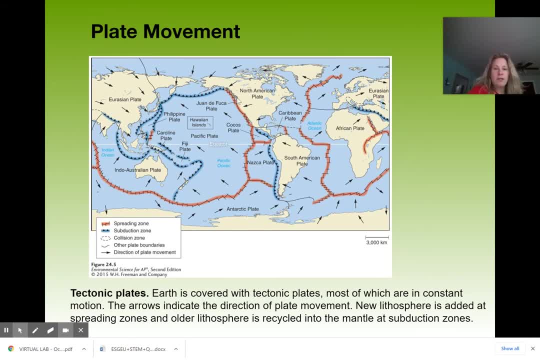 us the most for us in California is, in Northern California especially, is the Juan de Fuca plate, So this little tiny plate up here, And it's the cause of earthquakes that happen off of Eureka and Crescent City, So any earthquakes that we find happening there and Eureka often. 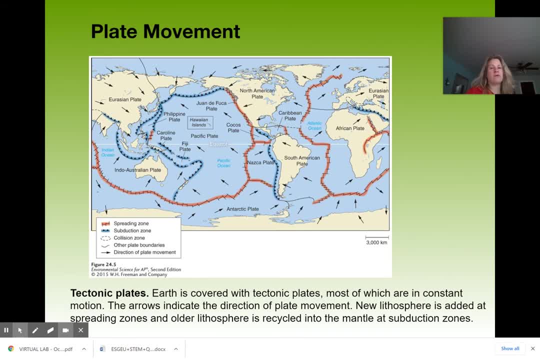 gets earthquakes, that's because of the Juan de Fuca plate. So the Juan de Fuca plate is subducting, meaning going under the North American plate. So that's creating the subduction zone, which is why we have volcanoes like Lassen and Shasta in. 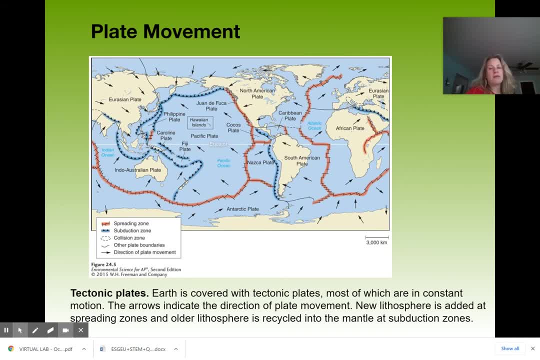 Northern California, But we don't have them in Southern California. And the reason we don't have them in Southern California is because the Juan de Fuca plate is up here only, And so down here we have sliding occurring, So the plates are like sliding past each other rather than going. 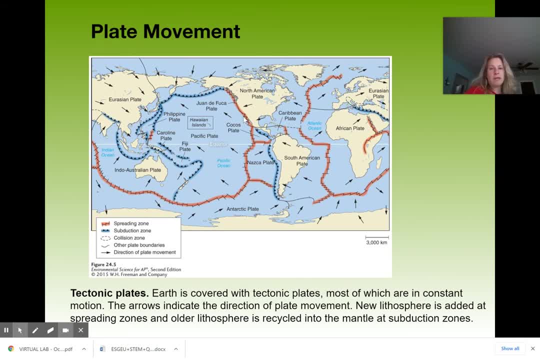 under, And so that would be the Pacific plate sliding along the North American plate, which is our San Andres plate. So that's why we have volcanoes like Lassen and Shasta in Northern California. So this is a different type of fault. It's sliding, It's a transform boundary, And so 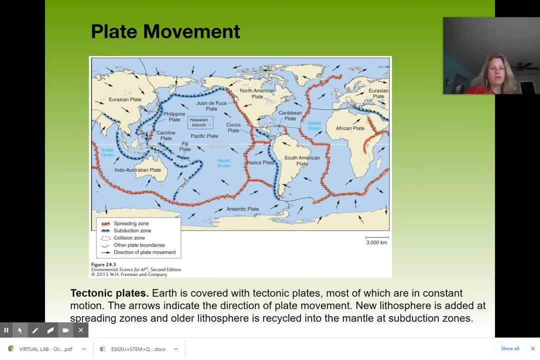 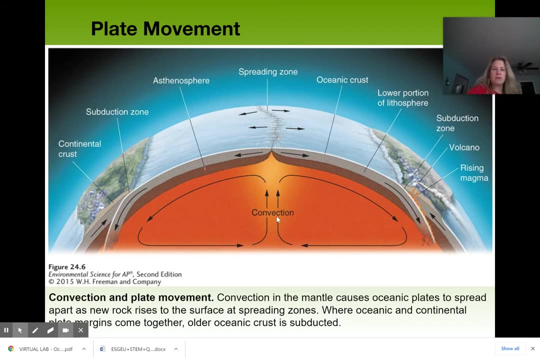 it's not creating volcanoes. Only the convergent boundary, which is the Juan de Fuca plate, is creating that, And you can see these little arrows are showing the movement of these plates all around the world, And that's plate tectonics. All right, So here is kind of a what's happening. 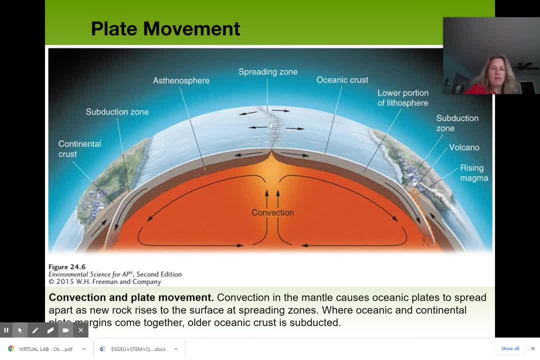 So mantle is convecting And we've got this plate spreading, which is a divergent boundary, And then we've got the plate moving this direction And eventually the earth is not getting bigger, So eventually the plate is going to subduct. 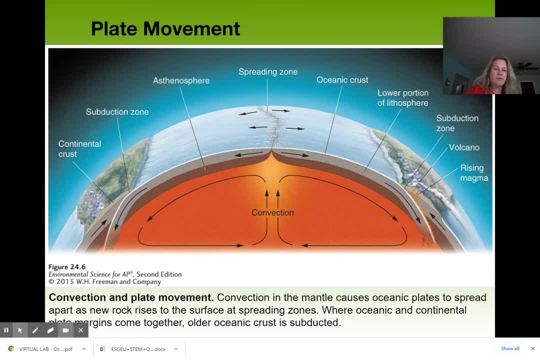 meaning going underneath. So this is a convergent boundary And this is where we get volcanoes or uplift like mountains, And then you can see over here, same thing is occurring. So we've got subduction occurring, We've got magma rising, We've got all of these volcanoes forming. 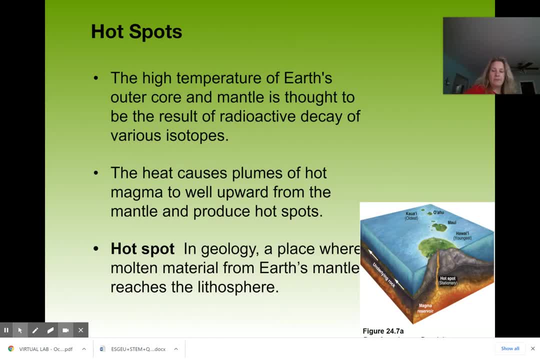 And that's plate movement, All right. So something else that we see here is called a hotspot, And so a hotspot happens in the middle of a plate, So it's not on a plate boundary, It is a volcano. We've got a couple that are 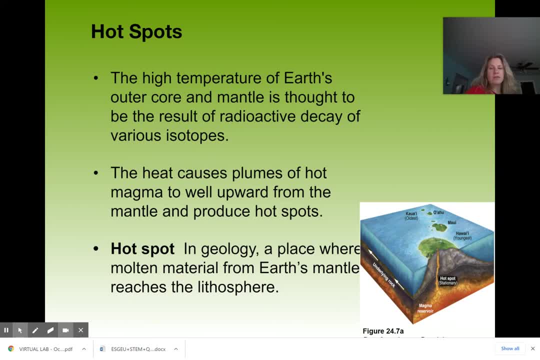 familiar to us. We've got Hawaii And then we also have Yellowstone, So Yellowstone is a continental hotspot. So hotspots are basically just an area in the mantle that is extra hot And it's melting through the plate. So as the plate moves along, the hotspot stays in the same place, So that 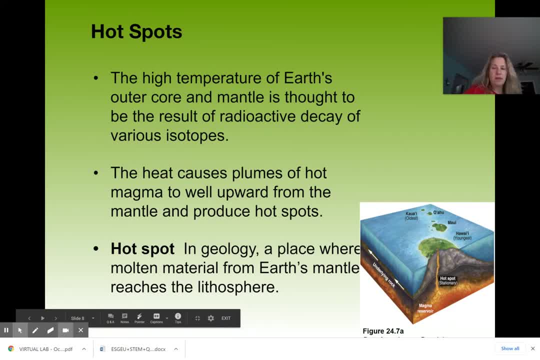 mantle that is extra hot, stays there And then the plate is moving across, And so you get chains of islands, like the Hawaiian islands, for example, And then we also get sometimes, like I said, a big volcano, which is Yellowstone, But mainly we get hotspots. So Hawaiian islands are formed by 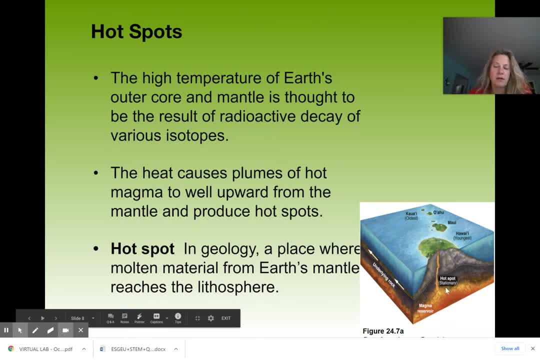 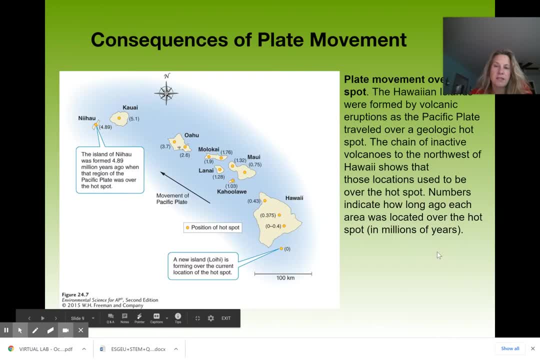 these hotspots Which are just a hotter layer in the crust, or in the mantle, I mean, And then, as the crust moves across, that magma seeps up through and creates these big, large volcanoes. All right, So if we 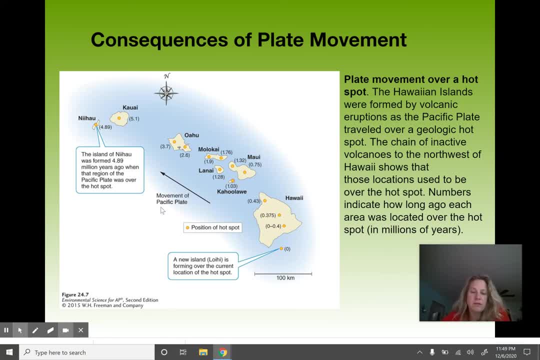 look at Hawaii. here we can see this is millions of years past. But the hotspot is here. It's kind of like right in here, It's kind of both. So these islands used to be on the hotspot But they have since moved on. They are not volcanic anymore. 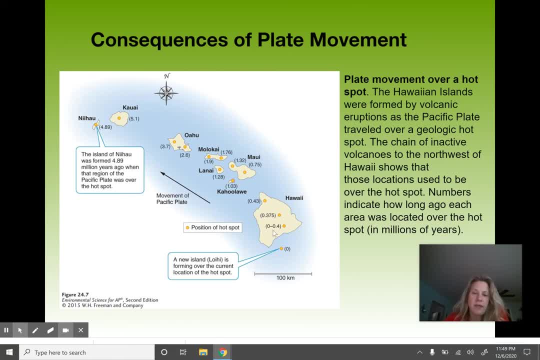 So they're not erupting. Hawaii is still erupting, And then we've got this new little volcano that is forming under the water, And so eventually, millions of years from now, it's probably going to be a new island, And so the direction of the plate movement is this direction, And so 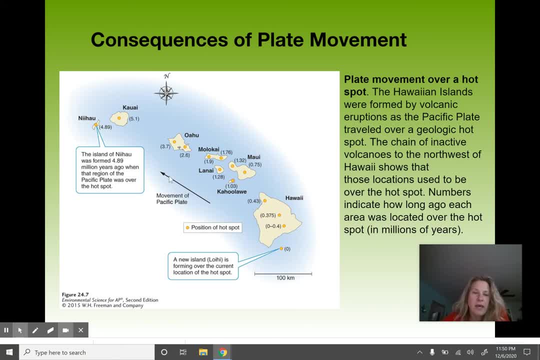 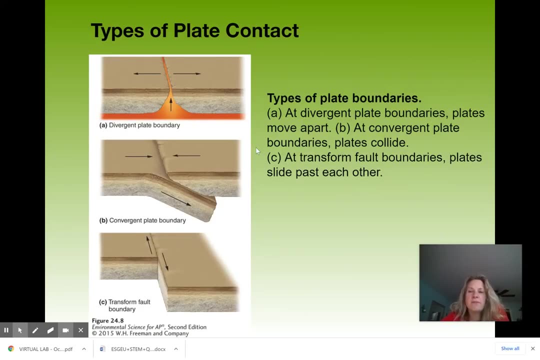 this is our oldest island that is above water, And this formed over this hotspot, And so this is our oldest one, This is our youngest one, And so it's moving in this direction, And that's how a hotspot works. All right, So there's three types of plate movements You might have. 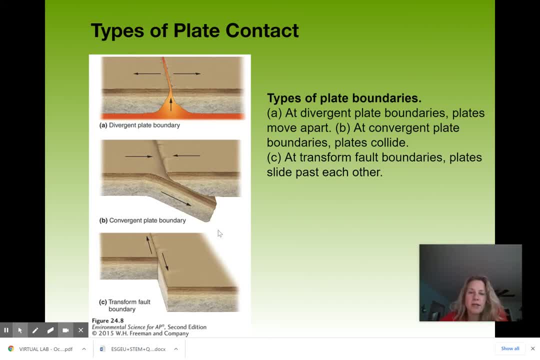 heard me mention them. We've got divergent, convergent and transform, So divergent is when they're moving apart, So that would be where the plate is splitting. And then we've got convergent, where they're coming together, So a plate is colliding with. 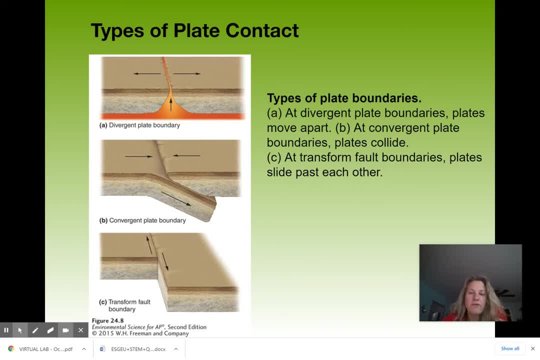 another plate And this is often where we get volcanoes, So we get volcanoes here too. Iceland is a great example of this, But here is like an example of Lassen or Shasta, So we've got melting occurring here And that. 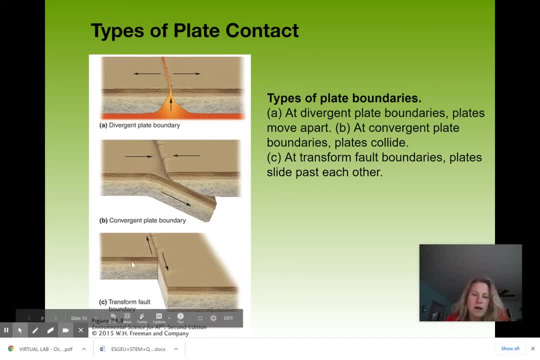 magma rises and forms the volcano here And then here we've got a transform boundary. So transform means it's just sliding past. There's no volcanoes that occur because there's no subduction, There's no magma forming. And those are our three types. 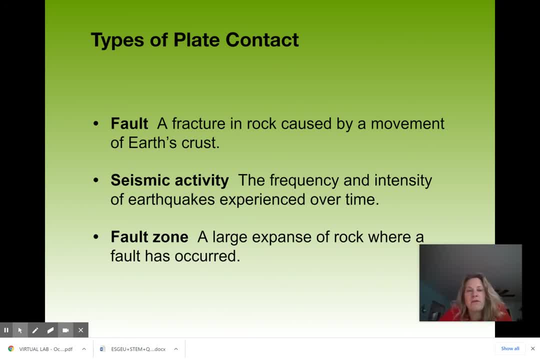 All right. So a couple other terms here. Fault is where you've got a break in the crust, And so that is usually where we find an earthquake, And then seismic activity is just the earthquake activity, So when the ground rumbles, that would be our seismic activity. And then a fault zone is just an area where we have 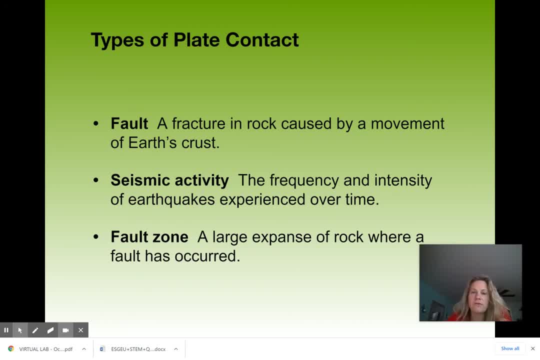 lots of faults. So California is a great example. There's faults all over the place, And that's because we are near a couple different plate boundaries. We're near the Juan de Fuca, which is convergent, And then we're also near San Andreas, which is transform, And then here's 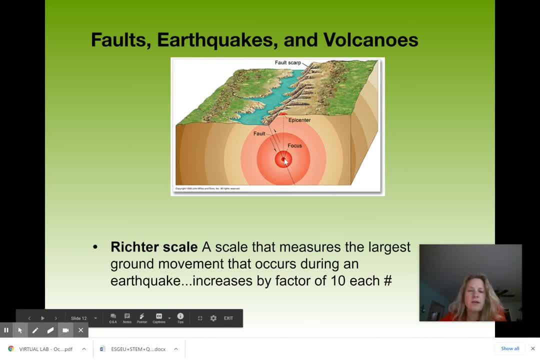 how an earthquake works. I mean, yeah, an earthquake. So here we've got the focus, And then the energy is radiating out in all directions, And so where it's going to radiate out and meet the surface first is going to be the epicenter, And then from 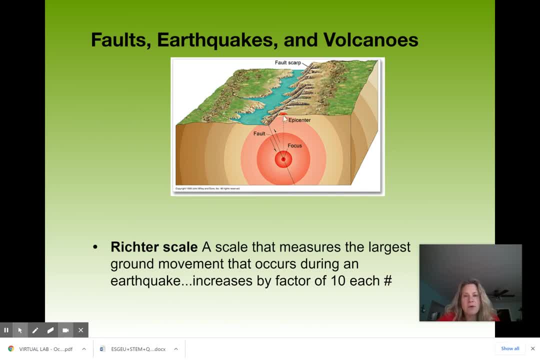 there. they might feel it out here, but it's going to be most intense here at the epicenter, And so when we measure earthquakes, we always talk about the epicenter. So where did it occur? Where was the epicenter? That's directly under the focus, So the focus is actually where it started, unless it 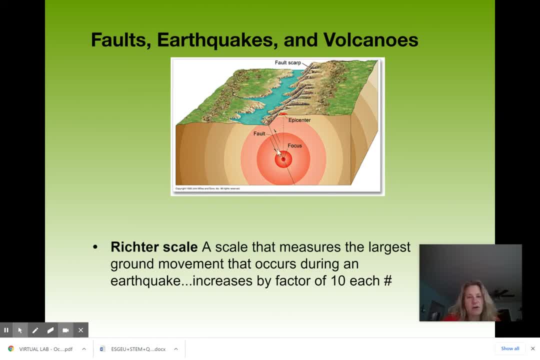 started on the surface, So it's going to be right under the focus And then from there it's going to be on the surface. But usually it starts on the fault line, which is not right on the surface, And then it radiates out in all directions like a ripple of a pond And that forms the earthquake on the. 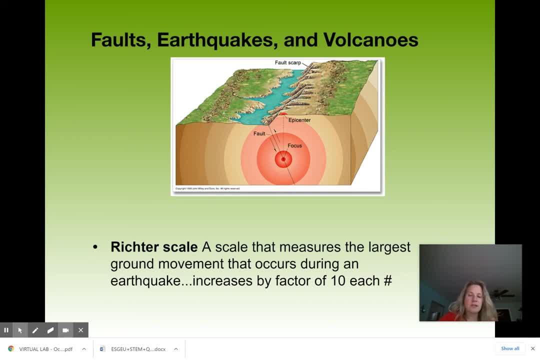 surface And the Richter scale measures that. So the Richter scale is increasing by factors of 10. So that means one on the Richter scale versus a. two is 10 times different. So you can see, that's excellent. I mean just you know. 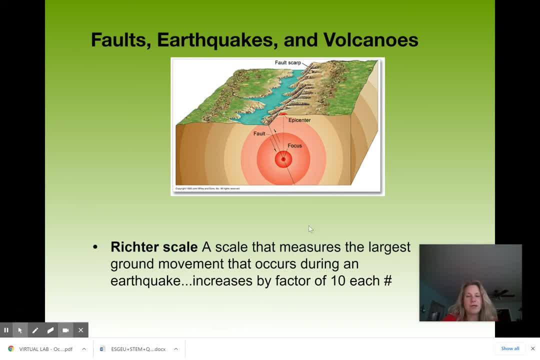 it's definitely like way stronger. So between like, when we measure a 3.2 versus a 3.8, that's pretty considerably bigger, even though it doesn't seem like it. But there are factors of 10, kind of like the pH scale, All right, And then here's where we have our plate boundaries, But we 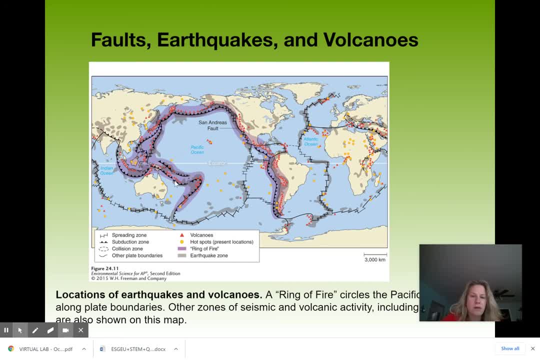 also. this is where it's showing a lot of different things. So it's showing plate boundaries, It's showing the types of plate boundaries And it's also showing where we have volcanoes, hot spots, And then this area here is known as the plate boundaries. So it's showing the types of plate. 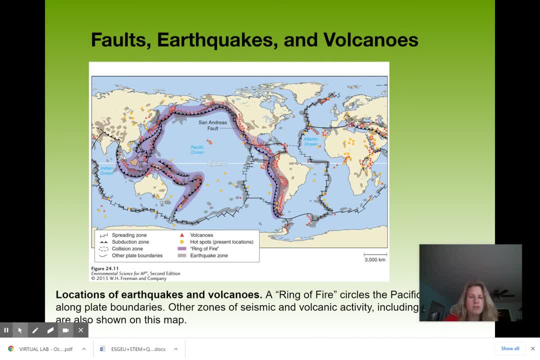 So notice how most of our volcanoes, our little red triangles, occur along this area. So this is all subduction. The Pacific Ocean is actually going underneath all the other plates And it's getting smaller And the Atlantic Ocean is divergent boundaries, So they're splitting apart And the 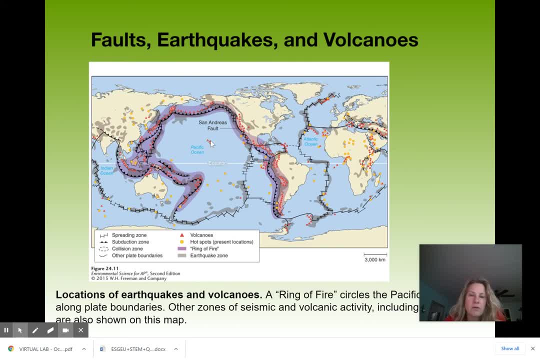 Atlantic Ocean is actually getting bigger. So here we've got our little islands, our Hawaiian islands, and that's formed by hotspot. But most of the earth, or most of the volcanoes along the earth or on the earth, is formed along this area, And so it's called the. 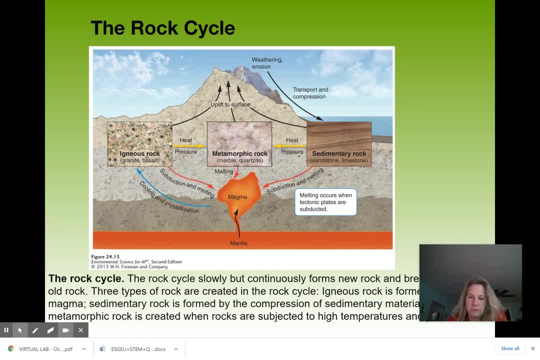 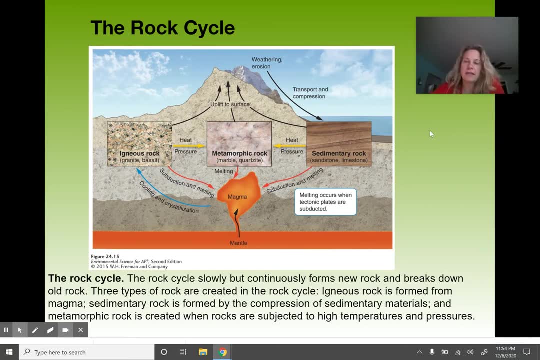 Ring of Fire for that reason. All right. And then the rock cycle. just you know, hopefully this is a review, maybe from junior high, or if you took earth science, then it should definitely be a review. But the rock cycle is igneous, metamorphic and sedimentary, And then basically, things are: 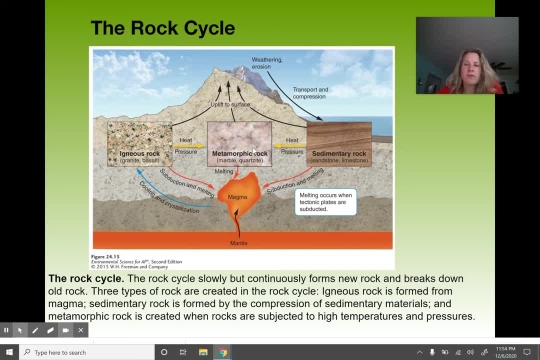 they're constantly changing. So a metamorphic rock is formed by heat and pressure. So if a sedimentary rock undergoes heat and pressure, it forms metamorphic. If an igneous rock undergoes heat and pressure, it forms metamorphic. If a rock melts and forms magma, 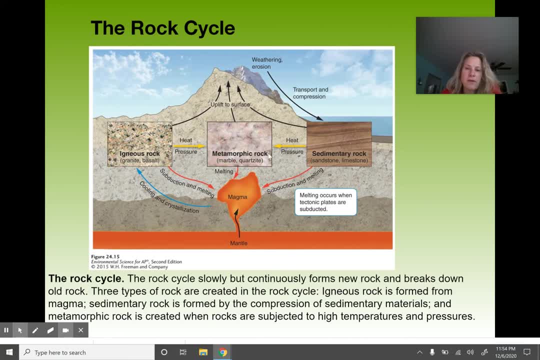 and then recrystallizes, it's igneous. If a rock crumbles and forms sediment and the sediment is squeezed together, then that's going to form sedimentary, And so sedimentary is formed by squeezing sediment together. Metamorphic is heat and pressure. 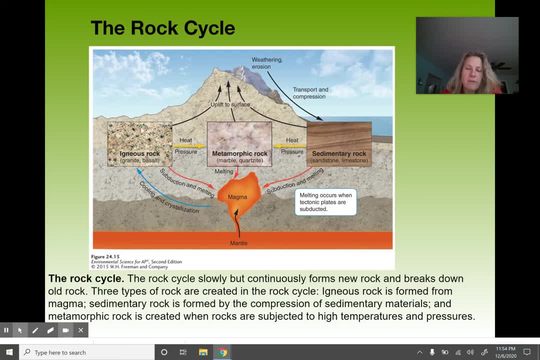 melting all the way though. So it melts partially but not all the way. And then if it melts all the way, it's an igneous rock. So things are constantly changing, So they're constantly changing. from these three types of rocks There's nothing really ever stationary Once these form. 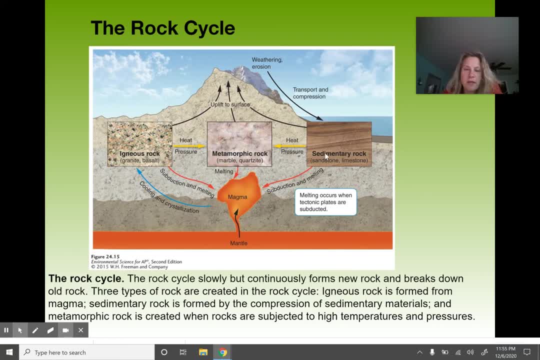 they're subjected to weathering, So they're going to weather and form sediment And then eventually, maybe a sedimentary rock and so on. All right, So these three types we've got- igneous, metamorphic and sedimentary to talk about, And then we're done. 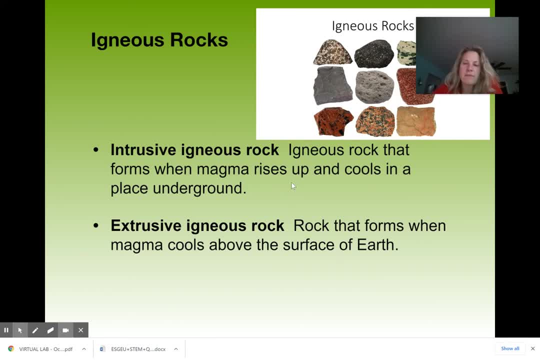 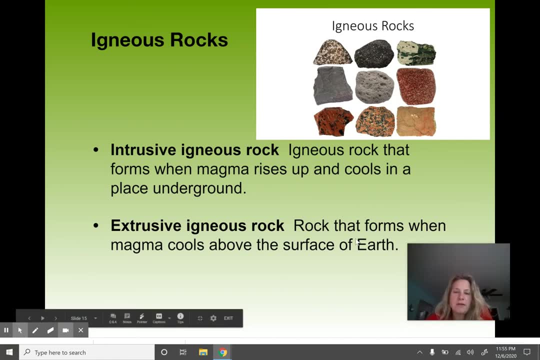 So intrusive igneous rock means that it forms inside the earth. So if we look at these pictures, we've got think about: intrusive is inside the earth, Extrusive is outside the earth. Extrusive is going to have no variation in color, whereas intrusive will. So if we look at these pictures, 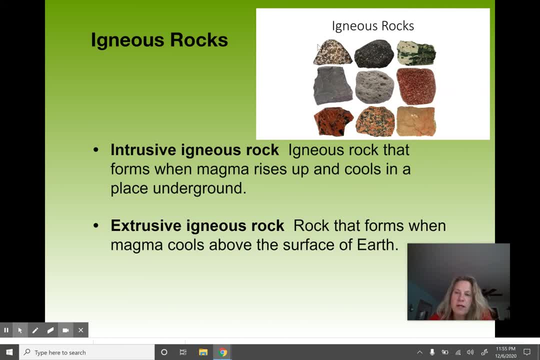 this first one is intrusive. So the reason I know that is because there's variation in color and those colors are minerals And so if it cools slowly it's going to have no variation in color. Then the minerals have time to join and meet up with the same minerals And then they form colors. 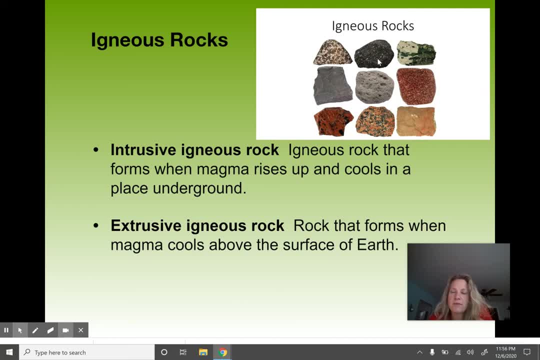 This is intrusive. I can see little white specks, So that would be formed inside. If you can see any kind of coloration at all, a variation, then it's intrusive. even if it's tiny, This one is intrusive, This one's extrusive, I see. no, I see like lighter color, but it's not a variation, It's. 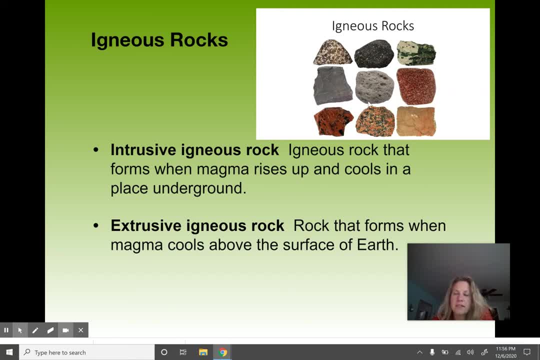 just lighter color. This has holes in it, but it's the same color. So if you look at these pictures, this is extrusive also. And then this one is intrusive, This one's intrusive, intrusive. This one's hard to see in this picture, but if I see different minerals in it then it's going to. 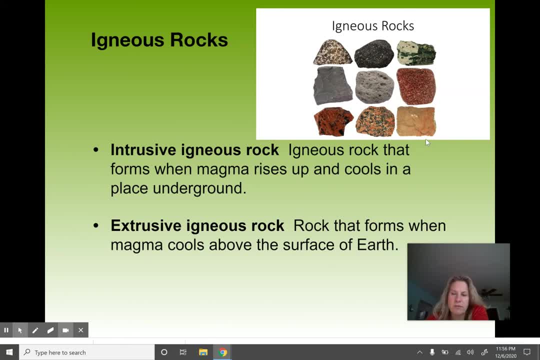 be intrusive, but I really don't. I see some coloring on it, but I don't think those are minerals, So I would say that would be extrusive. All right, So extrusive, no coloration variation, And then intrusive. you would see crystals or you would see a variation. 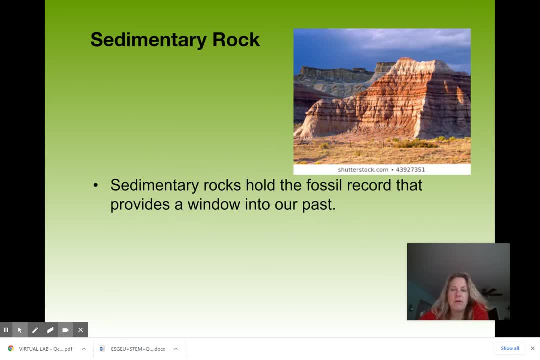 Variation in color, All right, And then sedimentary are formed from sediment layers. So here's an example, So we can see often really distinct layers like this, And so that's a sedimentary rock, And this is the only type of rock that we find fossils in, And that's because 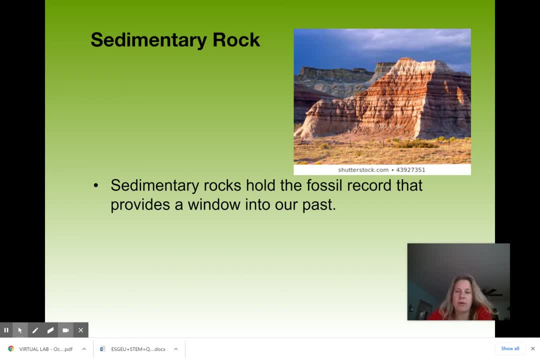 these are formed from sediment. The other two rocks are formed from heat and pressure or magma, So a fossil would be destroyed in any situation like that. So sedimentary rock- when it's just layers of sediment laid down on top of other rocks, that's a sedimentary rock And then sedimentary rock. 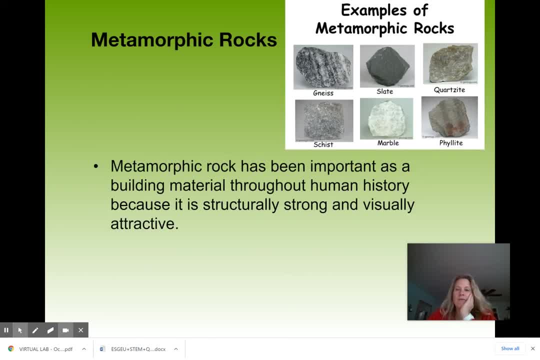 is where we would find fossils. And the last one is metamorphic. So metamorphic is a changed rock, So metamorphism means change. just like a butterfly metamorphosize, So metamorphic means that it's been changed. So here we've got some examples of metamorphic. So we've got gneiss, slate, quartzite. 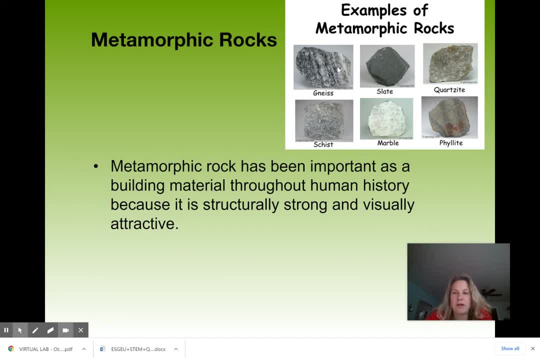 which is formed from sand. This is formed from shale, This is formed from a rock called gabbro And schist. marble and schist is a type of slate. It's just undergone more metamorphism. Marble is formed from limestone And phyllite is also formed from slate. So it goes: shale, slate, schist. 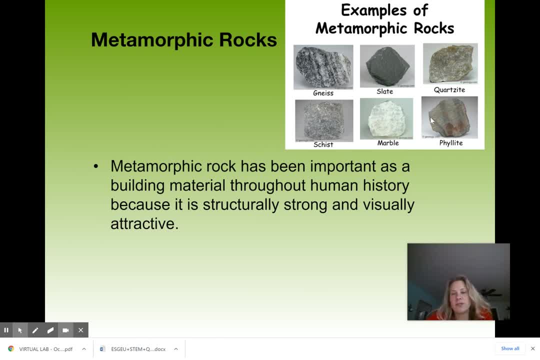 phyllite, And so those are how they form, in that order. So this has just undergone a lot more metamorphism than this has, And this has undergone even less than these two have. But these are all metamorphic rocks, So they're partially melted, So minerals don't melt at the same melting. 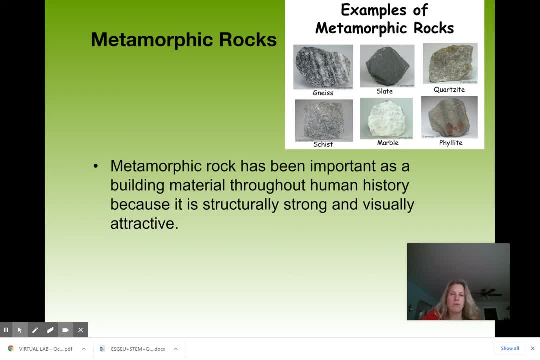 temperature. So if they partially melt, then only part of the rock, kind of like a chocolate chip cookie. if you have a, it's hot, the chocolate chips melt but the cookie doesn't. So it's kind of like that. So part of the rock will melt and then recrystallize and that forms a metamorphic. 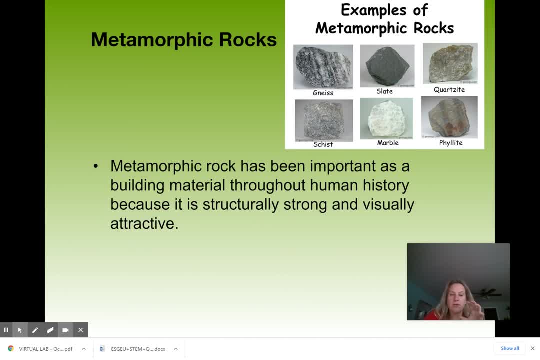 rock Or it's undergoing heat pressure. So if it's undergoing squeezing, then it's going to cause metamorphism. If you go out to Whiskeytown Lake and you look at the rock layers as you go out there and you drive and they've cut through the 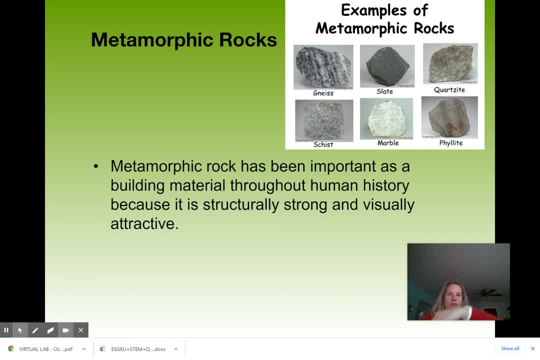 rock. you'll see the rock layers kind of do this like curving curvature And you can see it out shafted too, And those are. that's metamorphism. So metamorphism causes the layers, especially like sedimentary layers, to bend and buckle because it's undergoing heat and pressure. And that's it, So I will see you guys next time.